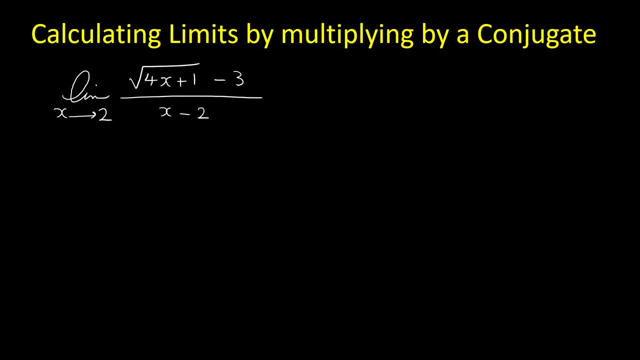 we need to find the value of the radical in the denominator and to find that we have to get rid of, have to multiply top and the bottom of this limit by the conjugate of the top. but maybe some of you are not familiar or you don't remember what is conjugate. 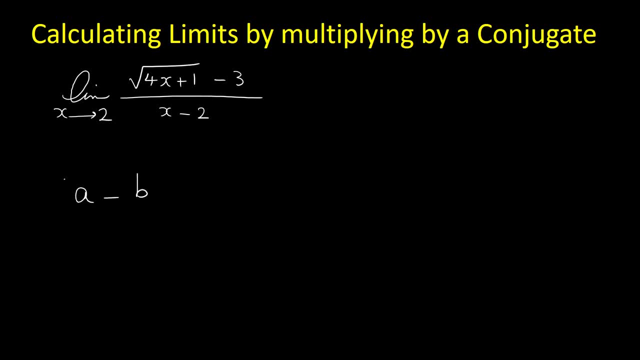 when we have a minus B, we say a plus B, conjugate of a minus B, or for a plus B, a minus B is the conjugate. so each of these expressions is the conjugate of the other one, and when we multiply them by together it equals a squared minus B. 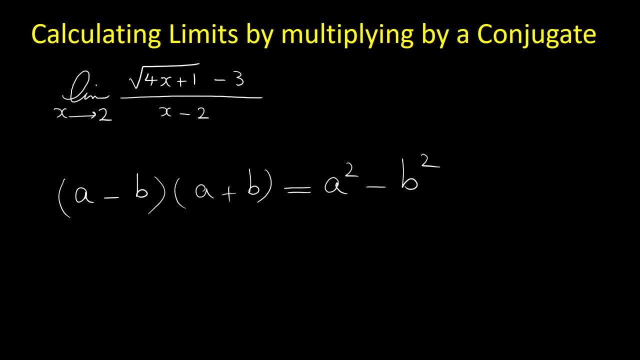 squared and because a and B is a squared, if they had radical. by these a squares we can get rid of those radicals. for example, suppose we have something like radical X minus 3. what is the conjugate of radical X minus 3? radical X minus 3. 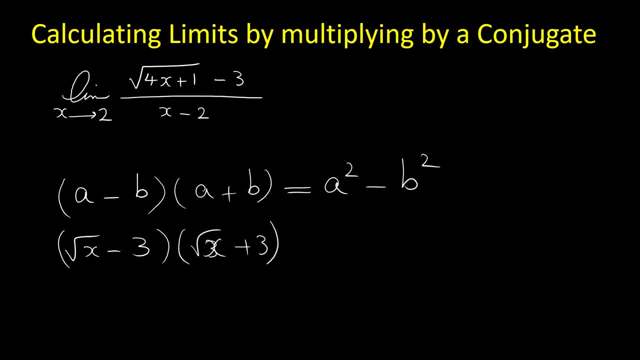 plus 3, and if we multiply them by each other, the answer is radical X to the 2 minus 3 to the 2, radical X squared is X and 3 squared is 9. as you see here, by multiplying radical X minus 3 by radical X plus 3, we could get rid of the radical. 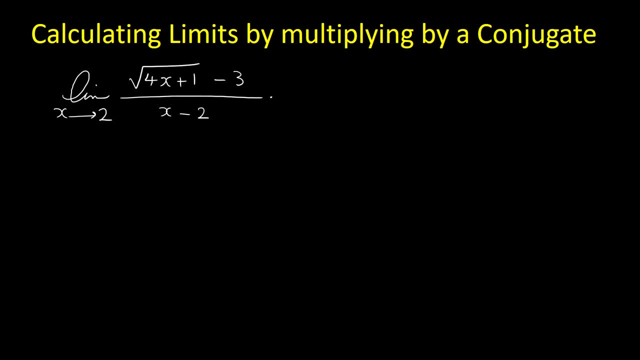 for finding this limit we have to multiply top and the bottom by the conjugate of the expression in the top and the conjugate of radical 4x plus 1 minus 3 is radical 4x plus 1 plus 3 over radical 4x plus 1 plus 3, why we have to. 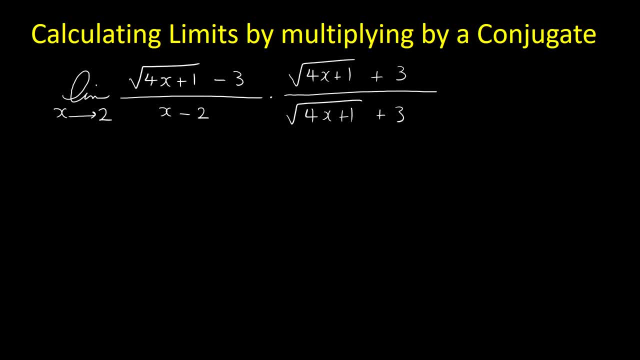 change the question. we want to keep the question as it was originally and by multiplying top and the bottom at the same time. by this expression, actually we multiply the limit by 1. note that this expression, all of these fraction, is 1. the top and the bottom are the same. so by multiplying the top and the bottom at, 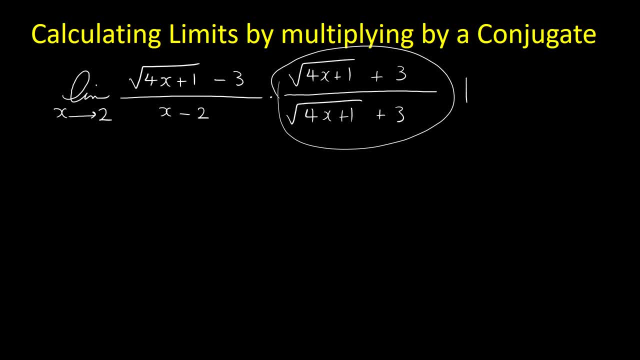 the same time by conjugate we are not changing anything. we keep the expression, the limit, as it was originally. but by multiplying by the conjugate we get rid of the radical. now if we multiply the expressions in numerator a minus b, if you suppose this a and this b, and a and b again a. 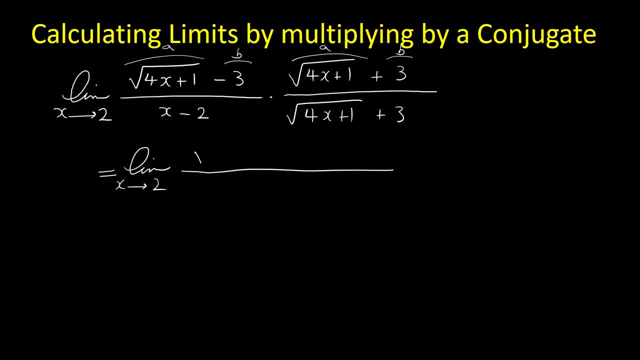 minus b times a plus b is a squared which cancels the radical of a, and you have 4x plus 1 minus b squared, and b squared is 3 squared or 9.. when you want to multiply the expressions in denominators, never multiply the expressions in the denominator and distribute them, just puts. 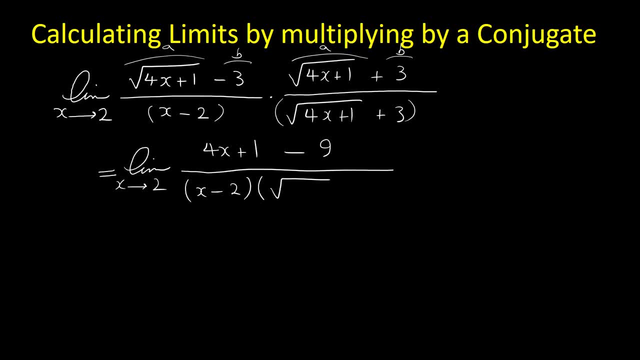 brackets around them, like i am doing here, and leave them in this form. don't distribute x minus 2 in the second bracket. now, if we look at the top, we have 4x minus 8 and in the bottom we have x minus 2 times. 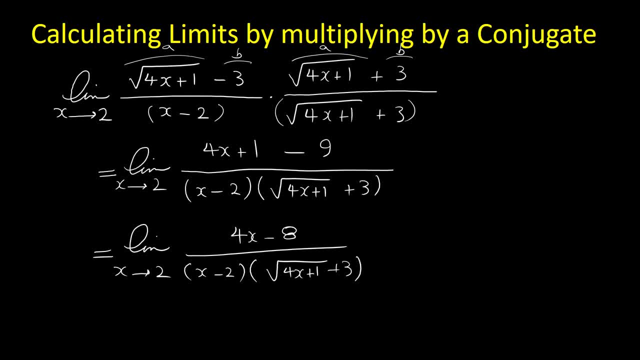 a square root of 4x plus 1 plus 2.. in the expression 4x minus 8, easily you can see that you can factor out a 4 and if you do so we have 4 bracket x minus 2 over x minus 2 times by radical, 4x plus 1 plus 2.. 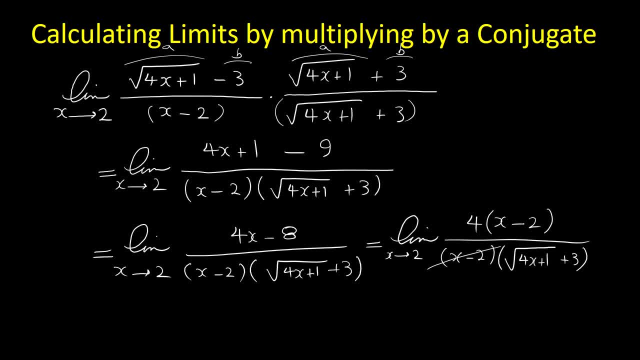 now you can see that we can cancel the term radicalization. common factor between the top and the bottom, which is X minus 2, and we have limit of X approaches 2. in top we have 4 and in bottom we have radical 4x plus 1. 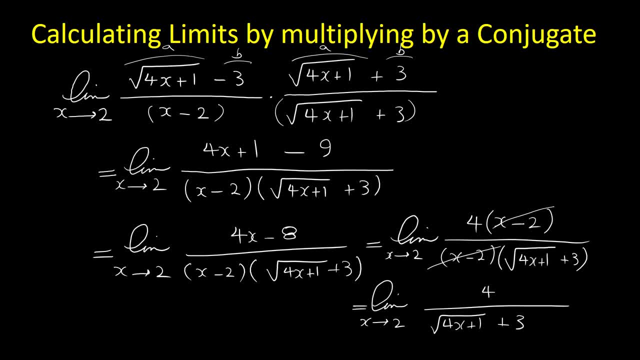 plus 3. now if you plug in 2 4 times 2 is 8 plus 1 is 9. radical 9 is 3 plus 3 is 6. 4 over 6 is 2 over 3. so the value of this limit is 2 over 3. limit of radical. 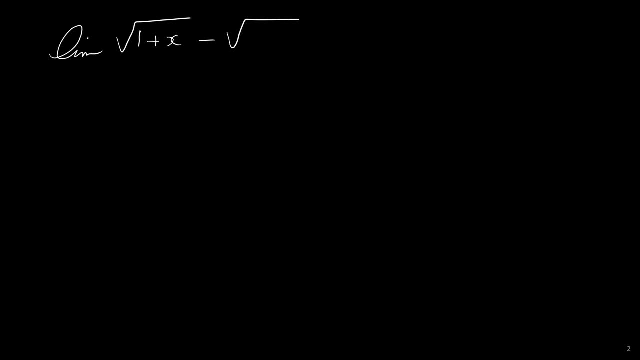 1 plus X minus radical, 1 minus X, all over X as X goes to 0 again. if you plug in 0 for X in top and the bottom, you get 0 over 0, which is in indeterminate form. so by direct substitution we cannot find this limit. we have to use conjugate method to find. 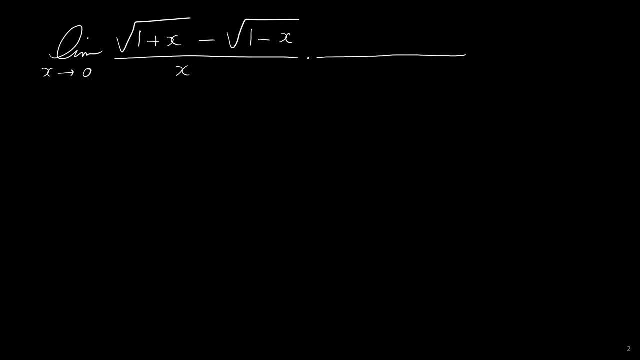 this limit. we multiply top and the bottom by conjugate of numerator, and the conjugate of numerator is radical- 1 plus X plus radical 1 minus X. and we multiply the bottom by the same thing. now we have 1 plus X minus 1 minus X in top. don't forget to put bracket around 1. 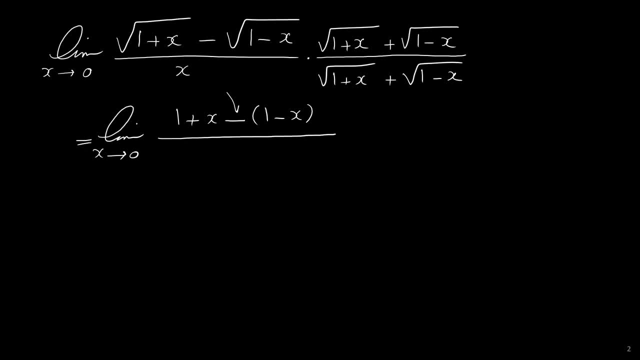 minus X, because this minus is for all of 1 minus 6, not only for 1, and in denominator we have X bracket: radical 1 plus X plus radical 1 minus X. if you simplify numerator, 1 minus 1 cancels and X minus minus X is actually X plus X. so 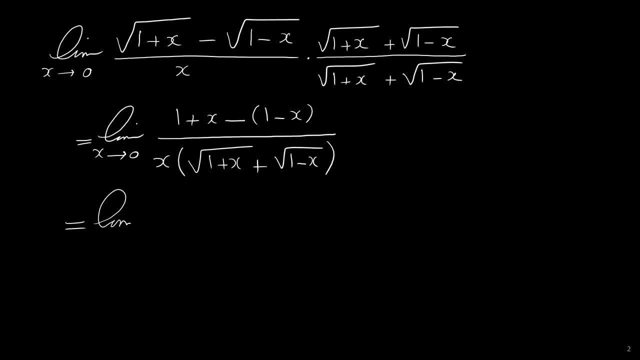 in numerator. we have 2x limit. X approaches 0 to X over X bracket. radical 1 plus X plus radical 1 minus X. if you cancel X from the top with X from bottom, we have limit of 2 over radical 1 plus X plus radical 1 minus X. now if you plug. 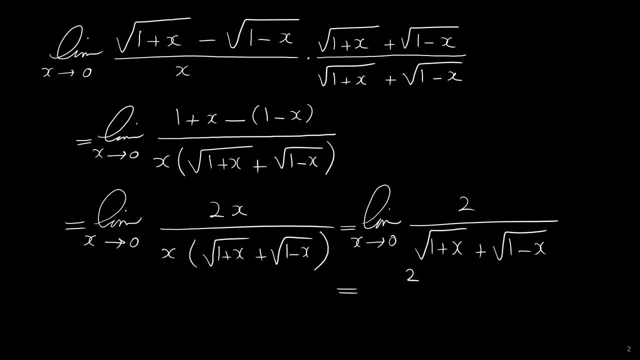 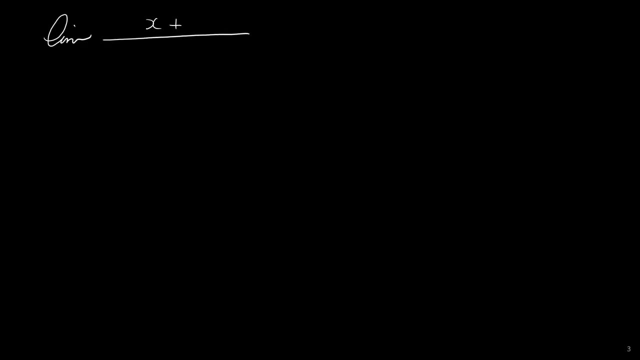 in 0 for X, you get 2 over radical 1 plus radical 1, 1, which is 2 over 2 or 1 limit of X plus 2 over radical X. 2 plus 5 minus 3, X goes to negative 2. if you plug in negative 2 in top and the bottom easily, you can see. 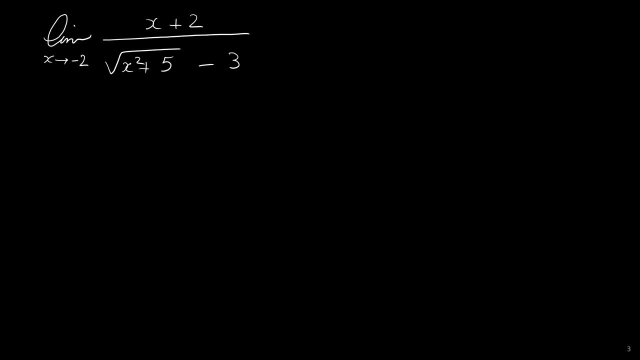 that you get 0 over 0, which is an indeterminate form. so direct substitution doesn't work. for finding this limit we have to multiply top and the bottom by the conjugate of denominator to get rid of radical in denominator. so we multiply top and the bottom by the conjugate of denominator. 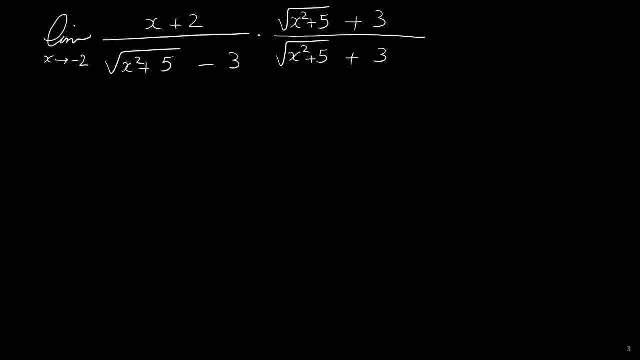 which is radical X 2 plus 5 plus 3. so by doing so we can get rid of radical in numerator. we have x plus 2 times radical X 2 plus 5 plus 3 and in the bottom radical in of top of x 2 plus. 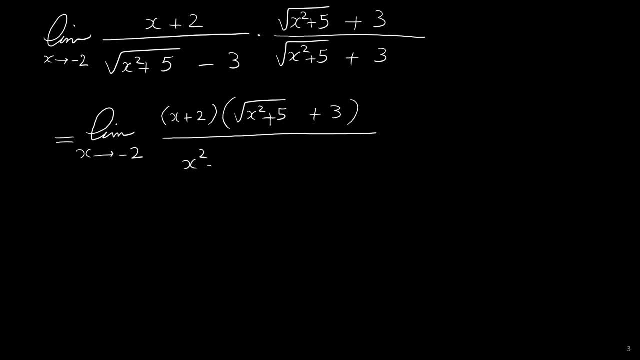 5 goes away and x 2 plus 5 remains minus. don't forget to s squared 3, and you get 9.. If you simplify x2 plus 5 minus 9 in denominator, you have x squared minus 4.. 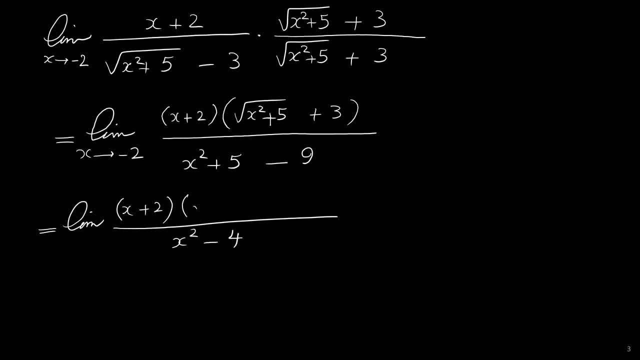 And in top we have the same thing. Now that we could get rid of the radical in denominator, we have to try to find a common factor between the top and the bottom. Because x approaches negative 2, we know that x plus 2 is the common factor that could be cancelled from the top and the bottom. 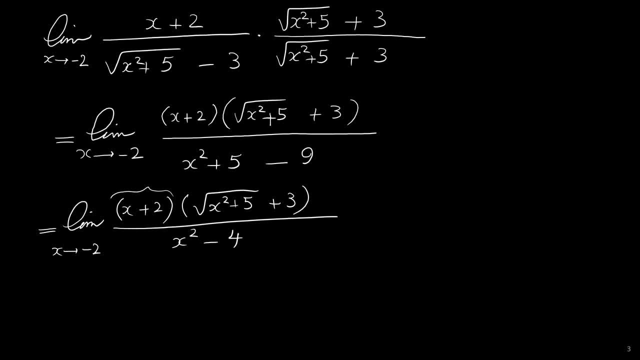 x plus 2 in the top is already here, so we have to have x plus 2 in denominator as well. If you attention easily, you can factor out x2 minus 4.. And one of the factors is x plus 2.. 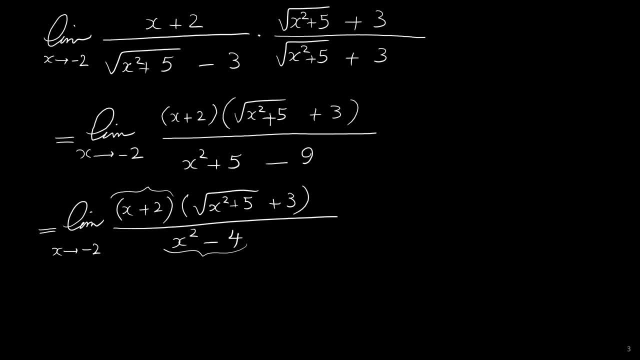 If you don't know why, when x approaches negative 2, we have to have x plus 2 as a factor between the top and the bottom of this limit. watch my video about finding of limits by factoring method. Now here, if we factor x2 minus 4 by difference of s squared's identity, 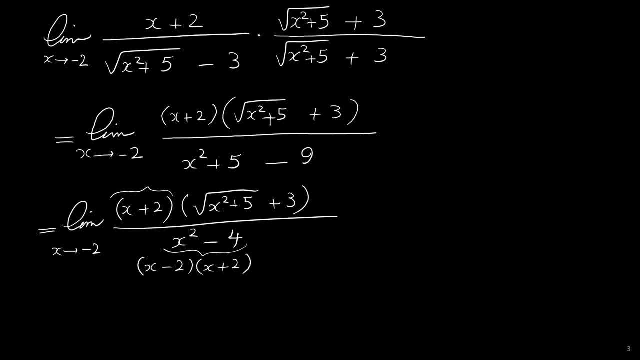 we can write it as x minus 2 times x plus 2.. If we cancel x plus 2 from the bottom with x plus 2 from the top, this limit equals to limit of radical x2 plus 5 plus 3 over x minus 2.. 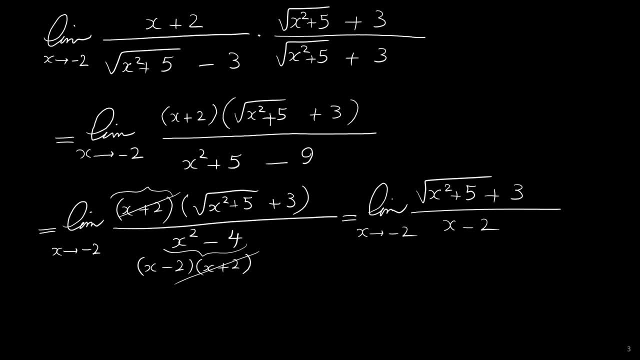 And x approaches negative 2.. Now if you plug in negative 2 in top and bottom, negative 2 squared is 4 plus 5 is 9,. radical 9 is 3 plus 3 is 6.. And in denominator we have negative 2 minus 2,. 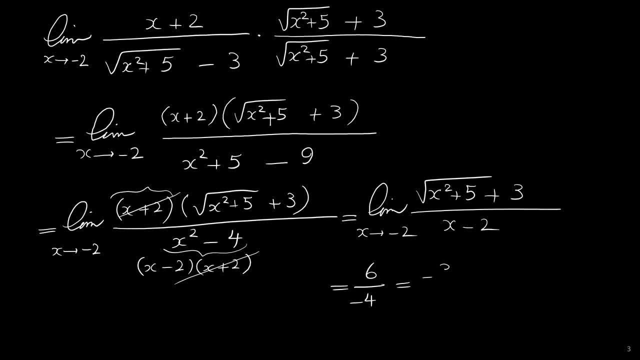 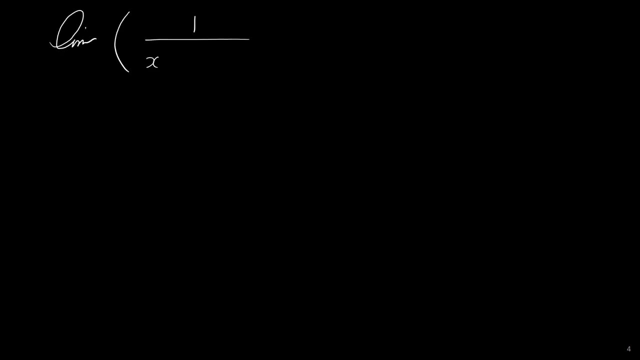 which is negative 4.. And if you want, you can write it as negative 3 over 2.. So this limit equals negative 3 over 2.. As the last example, let's find this limit: Limit of 1 over x: radical: 1 plus x minus, 1 over x. 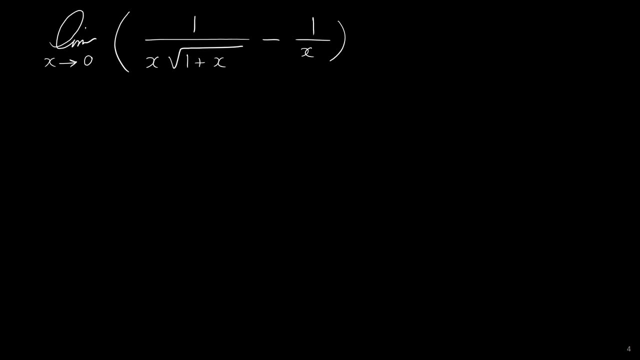 x approaches 0. If you plug in 0 in this limit, you will see that we cannot find this limit by direct substitution, because the limit is 0. Because this limit is actually in the form of infinity minus infinity, which is an indeterminate form. 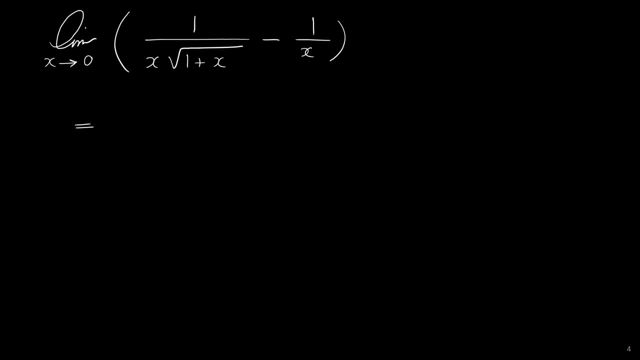 For finding this limit. first, we have to combine the two fractions. We have to do a common denominator to make the limit in fraction form one fraction. The question is: two fraction? by common denominator we make it 1 over x One fraction. similar to our previous examples. 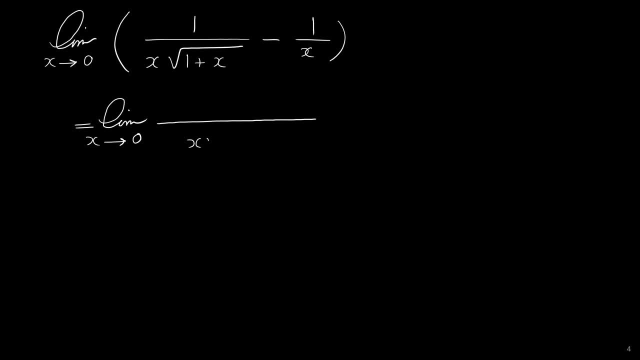 The common denominator is x- radical, 1 plus x And in the top we get 1 minus radical, 1 plus x. Some of the students at this step will become a bit confused because they think we have radical in the top and radical in the bottom. 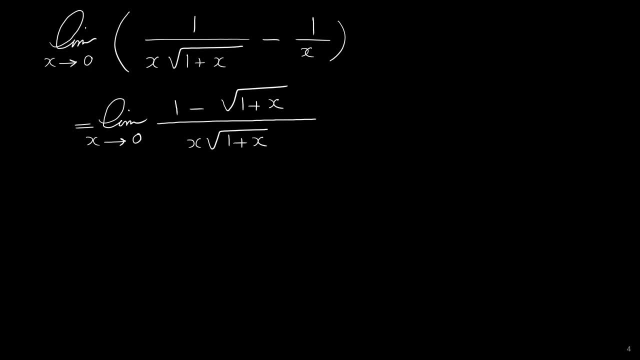 so we have to do conjugate for the top and the bottom at the same time. No, that's not true Here. for this example, we have to use the conjugate method only for top, And for the bottom we don't have any conjugate at all. 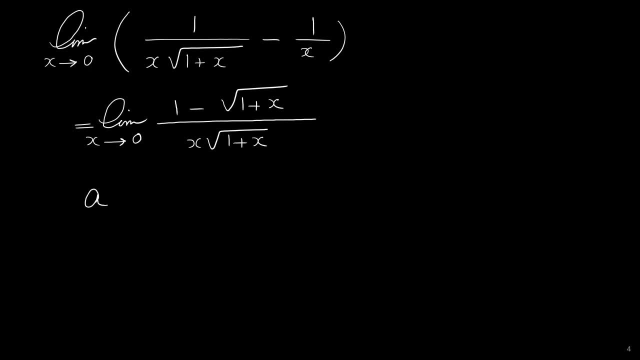 Let me remind you: conjugate means when you have two expressions like a and b, And between them is minus or plus. the conjugate of that is a plus b. In this example, in the top 1 is a and the radical 1 plus x is b. 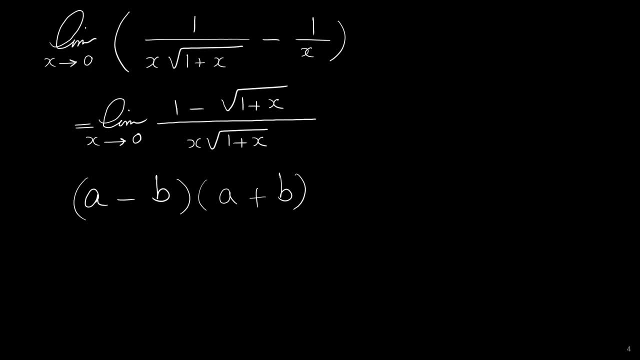 And between them is minus. So we have two terms with a minus between them, But in the bottom we have only one expression: x times radical, 1 plus x. We don't have two separate terms like a and b, With a minus or plus. 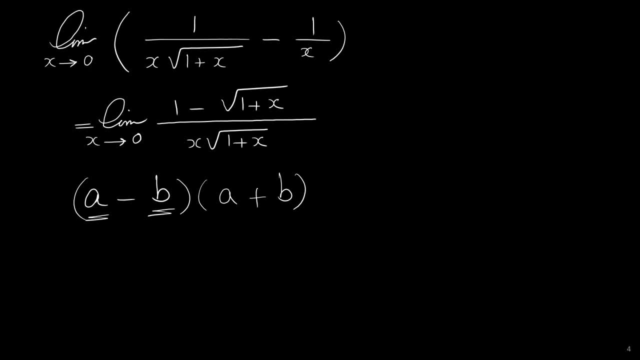 Between them, between x and radical. 1 plus x is multiplication. So multiplying the top and the bottom of this limit by the conjugate of denominator has no meaning at all. You can only multiply the top and the bottom of this limit by the conjugate of numerator. 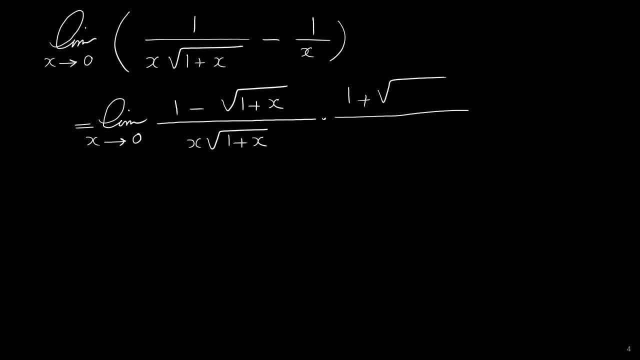 If we multiply top and bottom by conjugate of numerator, which is 1 plus radical, 1 plus x, we can get rid of the radical of numerator And we have 1 squared minus radical, 1 plus x squared, But radical 1 plus x squared is actually 1 plus x.